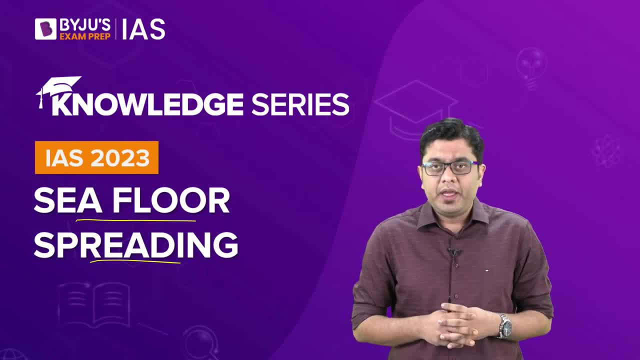 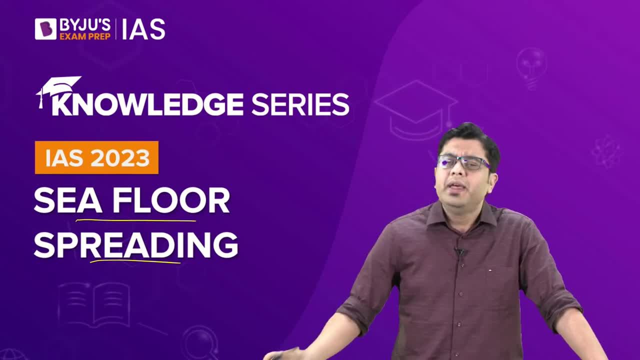 ends up indicating any kind of change. It was after Harry Hess in the early 1960s who provided this aspect of seafloor spreading. That is when we get an idea and we got an understanding about what really goes on at the ocean bottoms. So what is it exactly? If you take a look at the definition of this seafloor spreading, 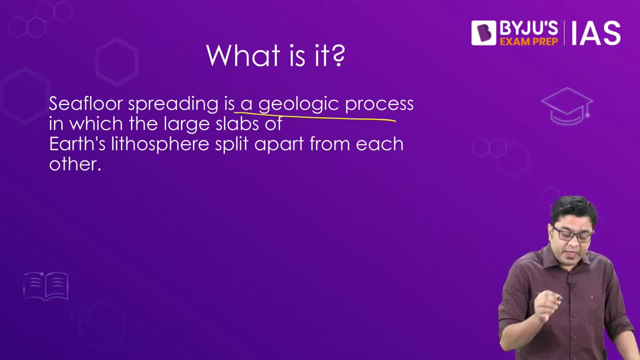 basically, it is a geological process in which the large slabs of earth's lithosphere split apart from each other. As simple as that. And where do they split apart from each other? At the region of the seafloor. So basically, during the Second World War, we had an unprecedented level of naval warfare. which was experienced across the globe. You had the powers such as Germany, who inculcated newer technologies, such as submarines and U-boats, by which they could carry out attacks to the unaware ships and vessels of United States, UK, etc. So countries such as United States, France, as well as Britain- they started developing. 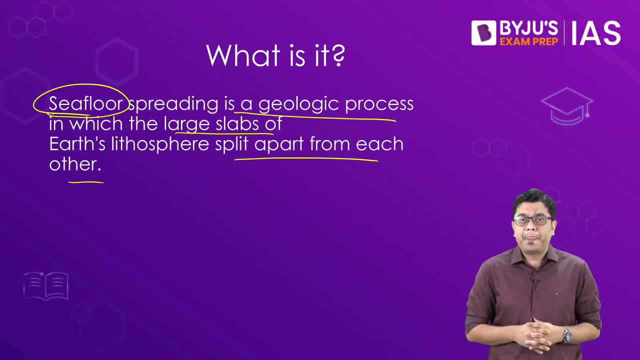 technologies in order to study the underwater region. Till that point of time, when mankind looked at the oceans, they looked at the ocean surface and always the perception was that the ocean floor is also going to be smooth and featureless. It was after the war ended that you had all these equipments which were lying idle. 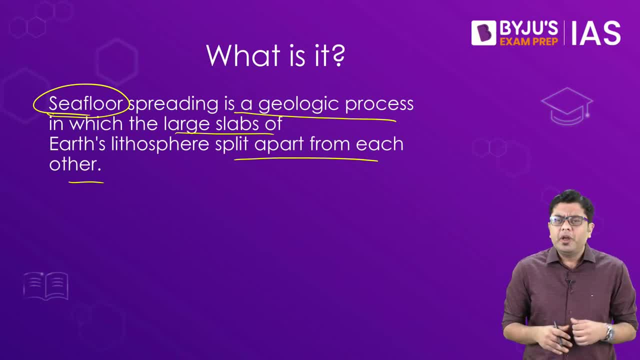 But then these equipments, which were used during the Second World War, was now being used in order to study the sea flow, And in this there was this American naval admiral in the name of Harry HS- Now Harry HS. he studied the ocean floors. and when he studied the ocean floors first, 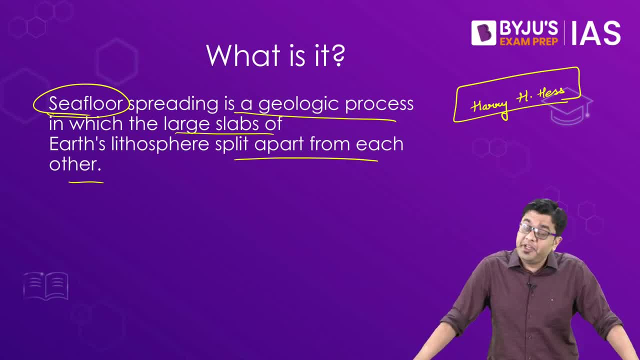 of all, he was surprised. He discovered various types of features that one could find on the ocean floor. It was the first time when a detailed study was carried out. He came across various different types of underwater features, such as sea mounts, goiarts. 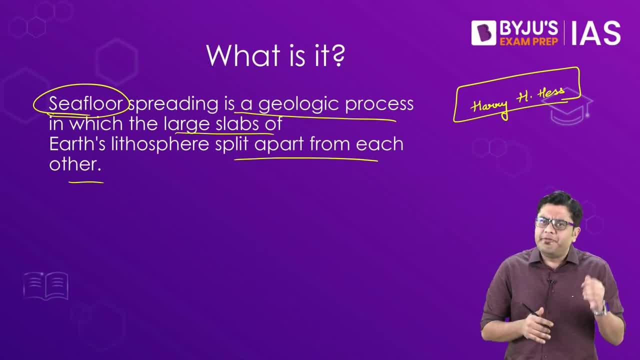 etc. Now, upon studying of the western part of North America, the sea floor along the western part, that is, the Pacific coastline, there he came across few of the interesting observations And based upon those sets of observations he propounded the sea floor, spreading theory. 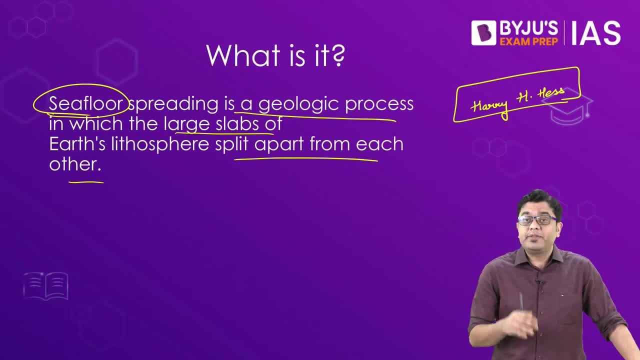 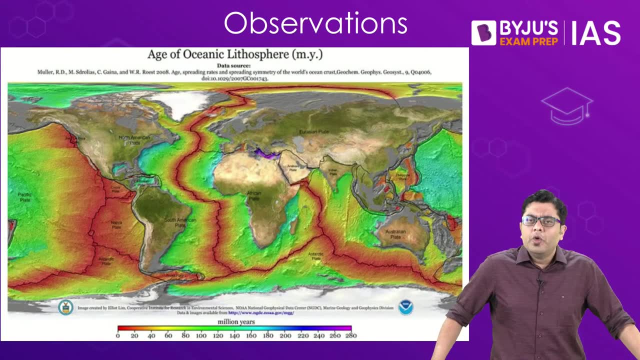 So what were the observations carried out by Harry HS on the sea floor? So one of the first observations and the most important observations that was carried out was regarding the age of the sea floor. While the continental rocks and the continental land masses, due to the help of geological 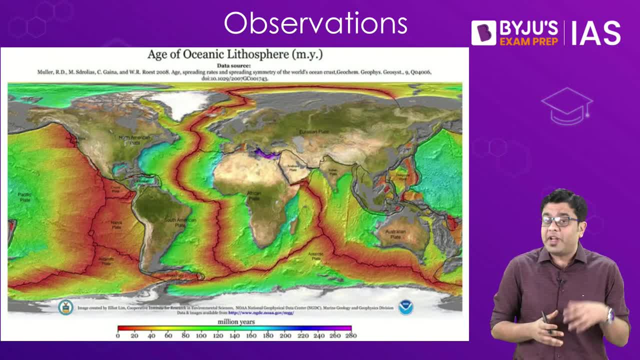 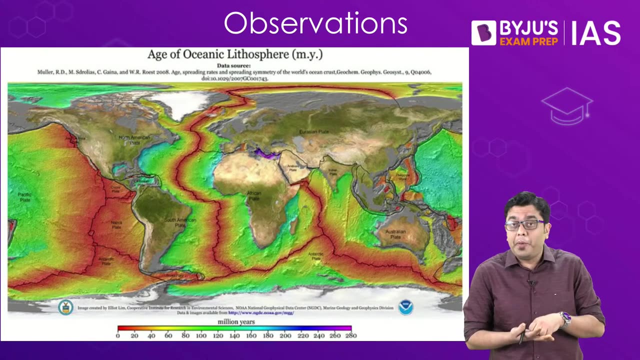 dating we could come at a conclusion that continental rocks and continental land masses were as old as three and three and a half billion years. But then the sea floor was much younger Sea floor there, even the sediments which were found at the bottom of the sea floor. 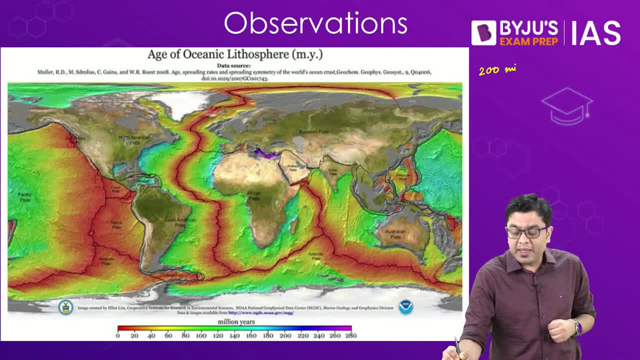 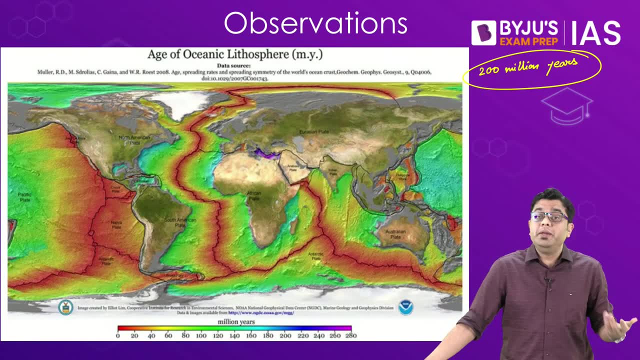 were not older than 200 million years. So this was the first puzzle which came up and which emerged before their very eyes: That how is it possible That? how is it possible That when, in certain areas of the continental land masses, we come across rocks which are 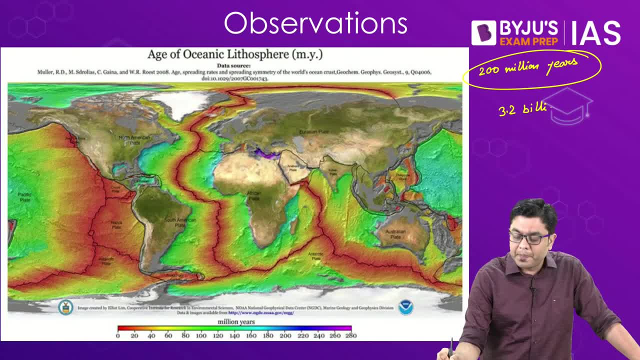 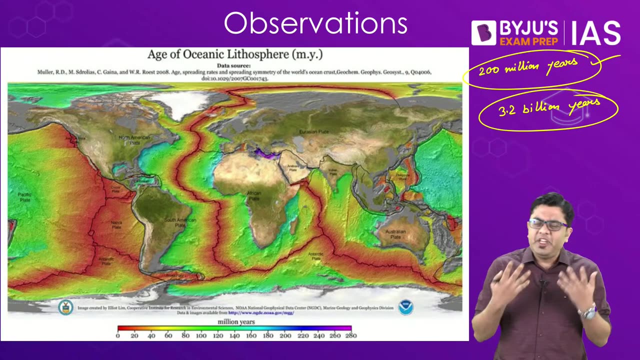 as old as 3.2 billion years. How is it possible that we have the oceanic bottom which is only 200 million years old? More particularly so, along the ocean bottom he came across certain features which now we refer to as mid-oceanic ridges. 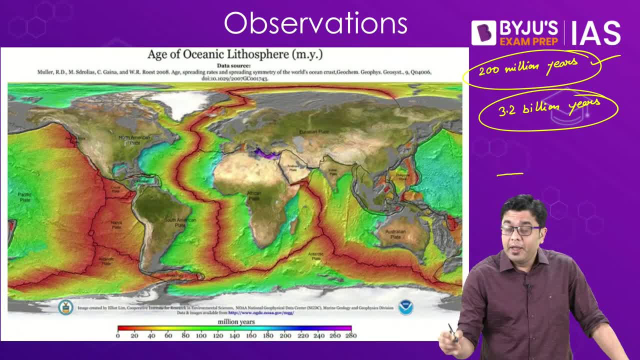 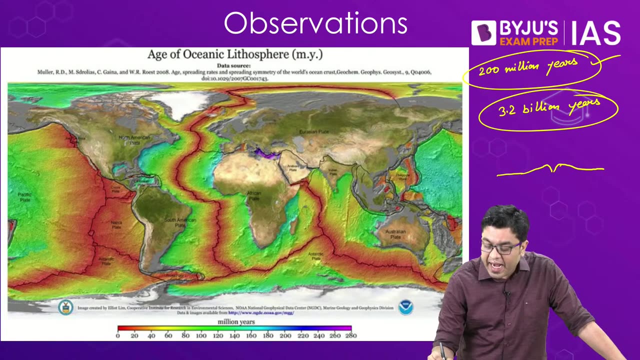 So at the ocean floor He came across a phenomena whereby along the ocean floor there was a kind of an uplifted land mass and a valley like portion at between. Now, this upliftment and this uplifted land mass had a height close to around 1 to 1.5. 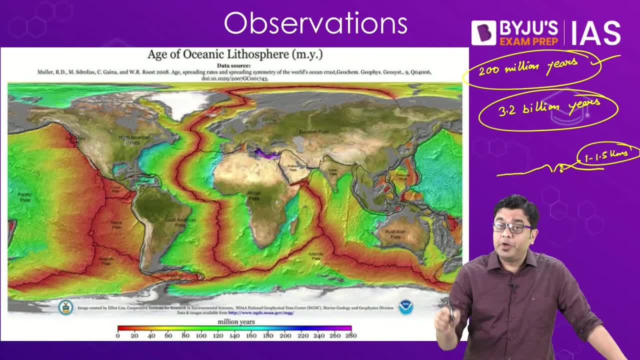 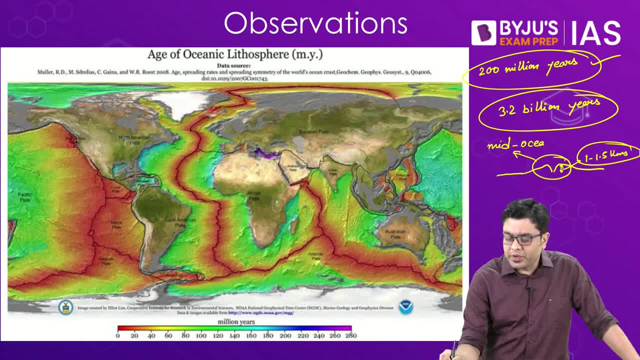 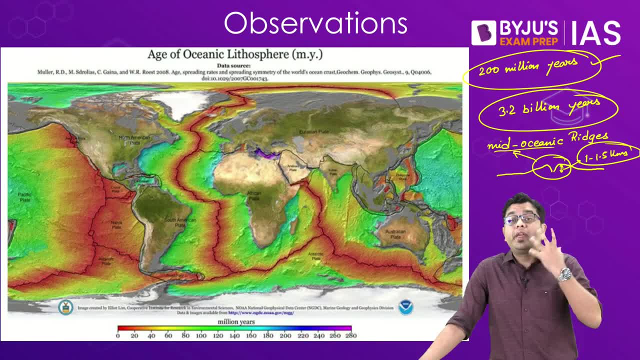 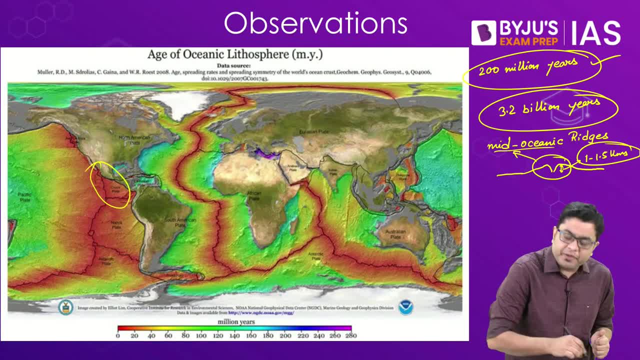 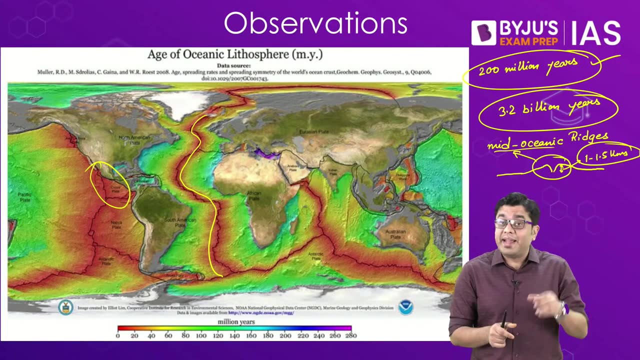 These mid-oceanic ridges were not only found along the Pacific coastline to the western part of North America, but they were found to exist in an entirety of the region, across the Atlantic as well, And furthermore, upon examination of the sediments and examination of the rocks along these mid-oceanic 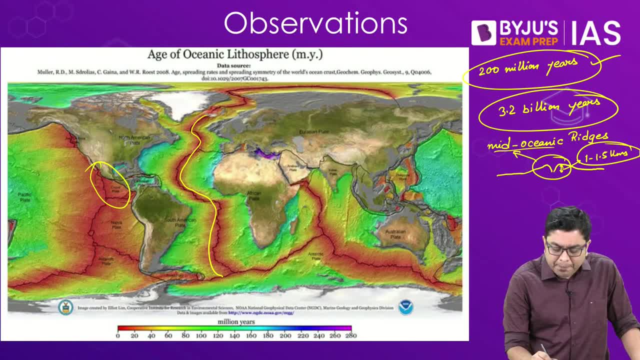 ridges. it was further found out that, basically, the portions which were closer to the mid-oceanic ridges, they were very, very new, whereas the portions which were further away from the mid-oceanic ridges, these were older. 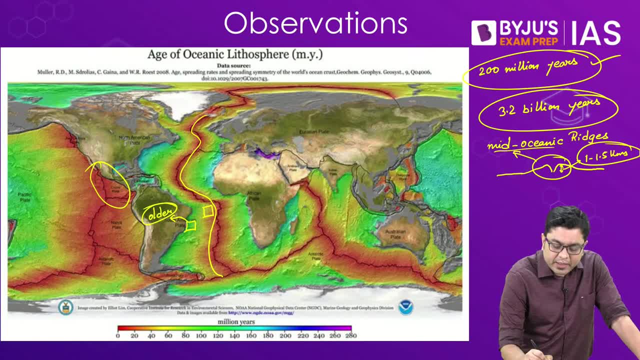 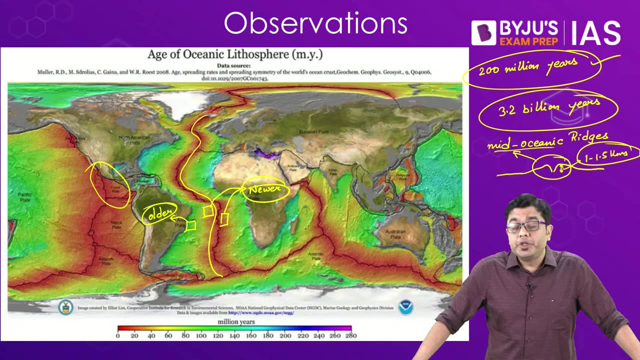 So these were comparatively older, whereas the portions immediately surrounding the mid-oceanic ridges, these were comparatively very new. Now This formed the base for the postulation of the theory of seafloor spreading. Now, by the time that Harry Ayers could propound the seafloor spreading, we had a convection. 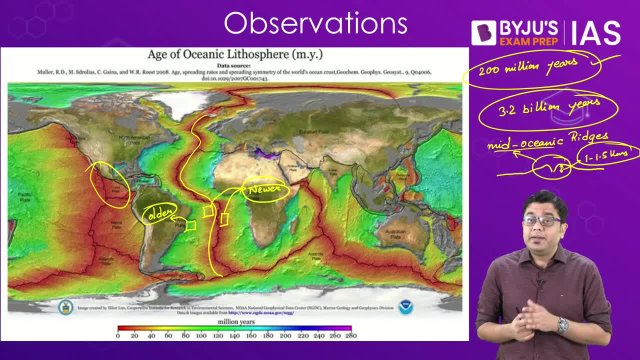 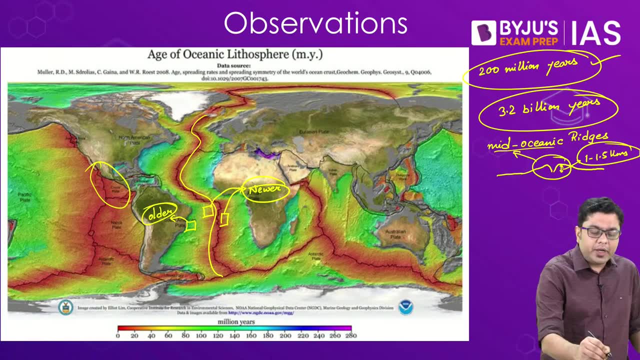 current theory which was provided in the late 1920s and the early 1919 as well, And that was the convection current theory which was postulated by Arthur Holmes. Now, Arthur Holmes, he provided us with a convection current theory. 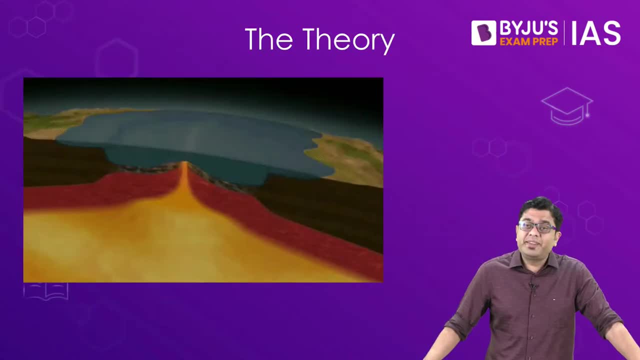 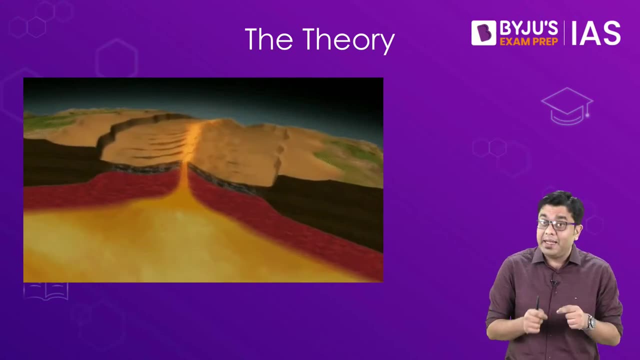 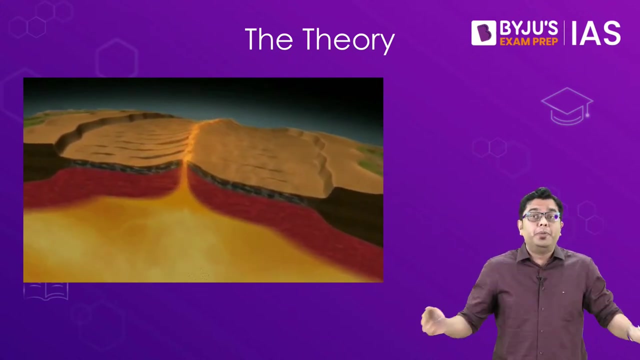 Now, what was this convection current theory? So, as per this convection current theory, due to immense amount of residual heat which is trapped still in the Earth's interior, significant amount of this heat escapes, and tries to escape, to the upper portion of mantle. 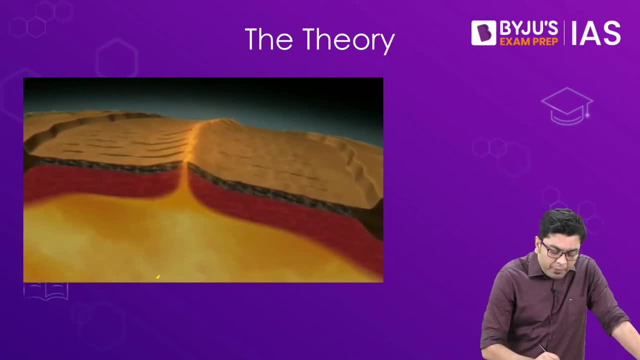 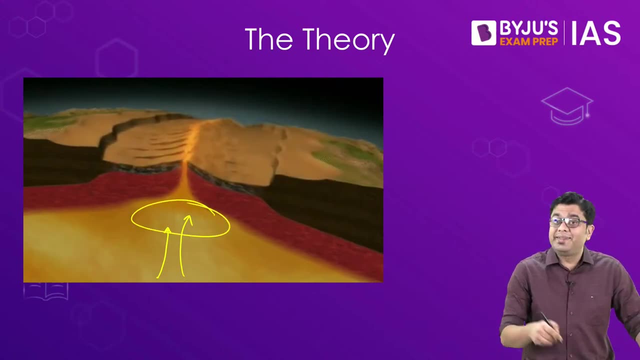 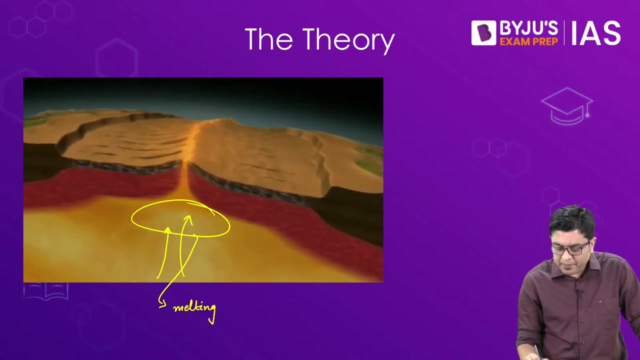 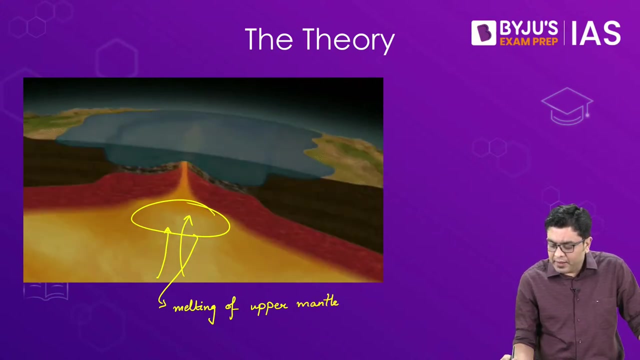 Now that excess amount of heat which comes from the lower layers to the upper portion of mantle, that heat leads to melting of materials in the upper portion of mantle, Melting of upper mantle. And this melting of upper mantle was largely supported by the continuous convection currents. 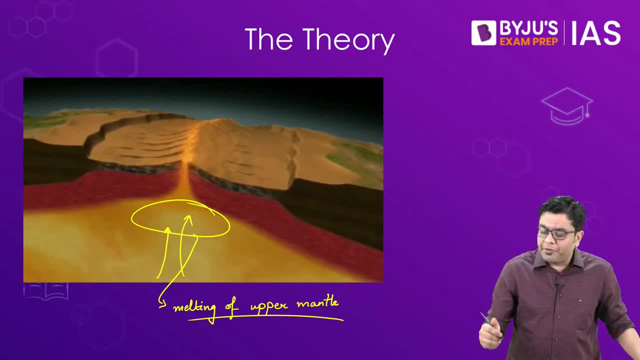 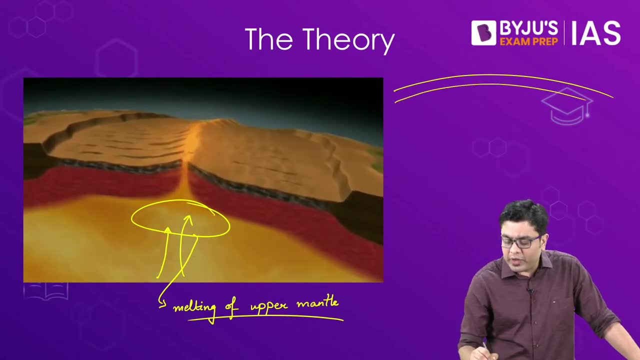 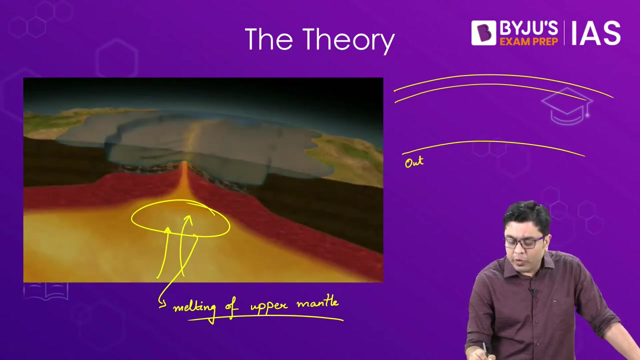 which persisted in the interior. So if you have to take a look, if you have to imagine This heat, This convection current theory is a very typical explanation of the convection current theory. So if you have a layer of this layer of deep upper BMC, which is an acidicатic layer, and 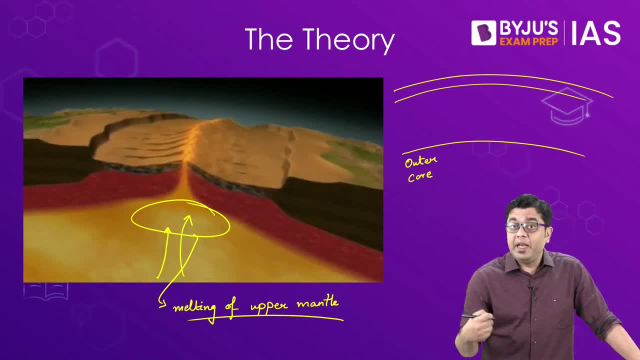 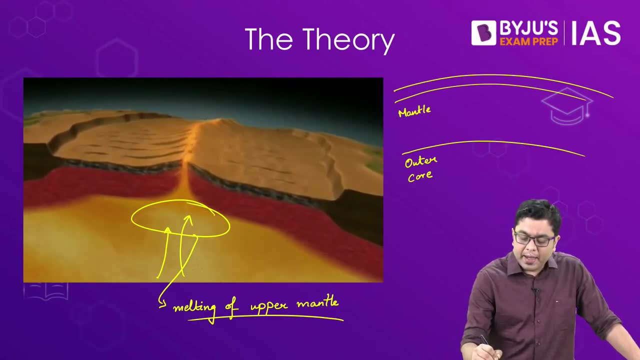 here this layer is a liquid layer. then in the lower layer on higher below is a cor theology state for this layer toなので conducting a convection current theory. Basically It is known that behind the layer of core of a mantle Has a molten outer core very intense state form. 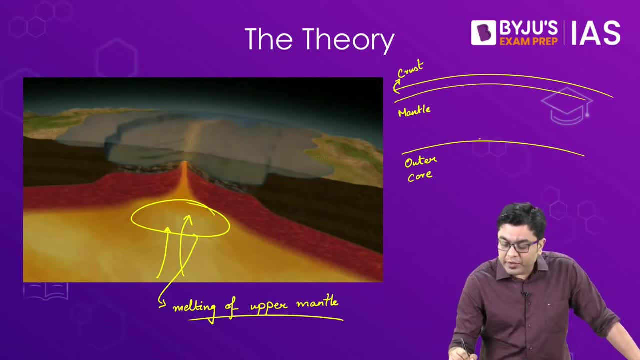 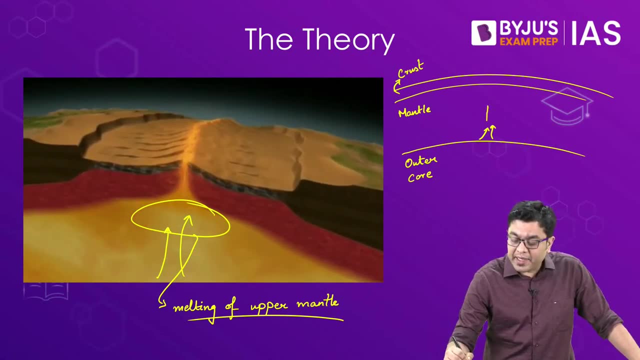 And the internal outer cor, the convection current theory, the heat which was provided, heat which was supplied from the region of the outer core, that heat sometimes traveled all the way through the mantle and then that heat diverged and also sunk down, creating a kind of a convection current. So this basic 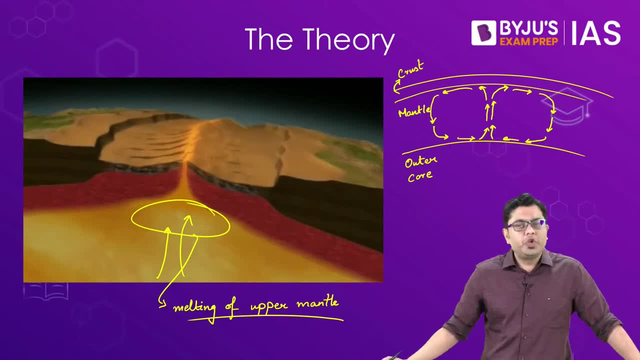 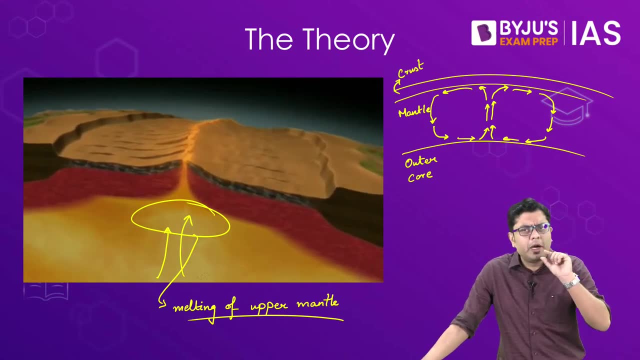 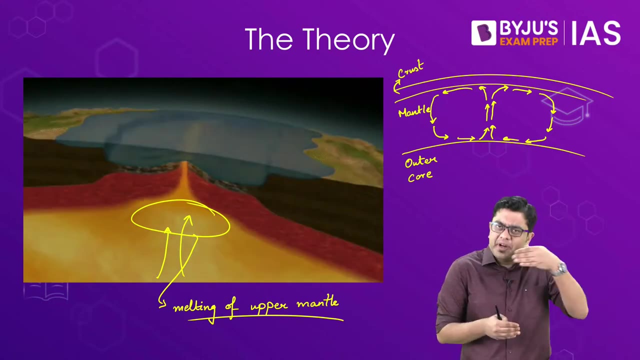 aspect of heat transfer was postulated by Arthur Holmes, and this was done in 1990 and 1920.. It was worked upon and tweaked upon in the early part of 1920s as well. So, based upon this postulation, it was further developed by Harry Hess, and Harry Hess said that as a result of this, heat which is produced, you have molten materials which start coming out from these mid-oceanic ridges, and mid-oceanic ridges are the regions of newer crustal formations. So newer crust is created where it gets created- at mid-oceanic ridges. 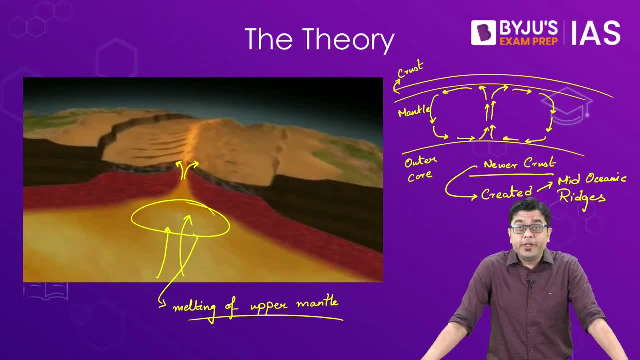 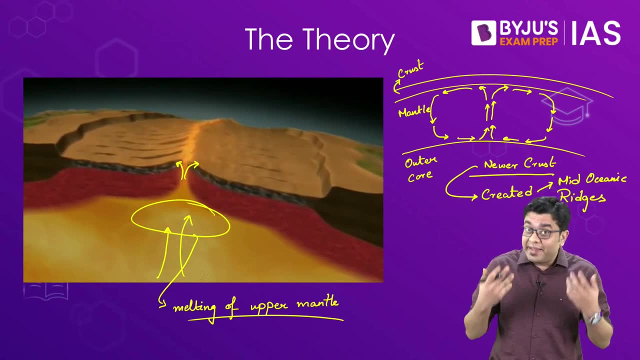 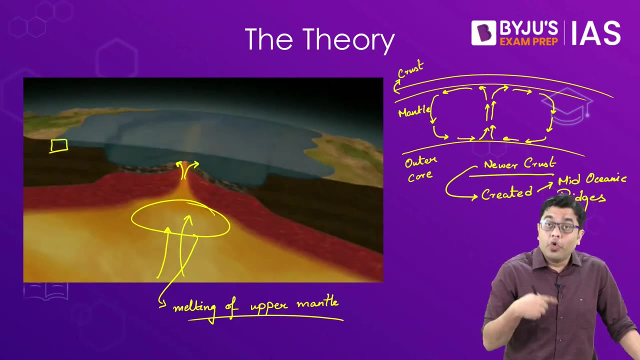 And it was basically postulated that, because the newer crust gets created there, that is what pushes the older crust aside, And this would be the reason why, as you move away from the mid-oceanic ridge, you would find older sediments and older rocks, whereas when you talk about the 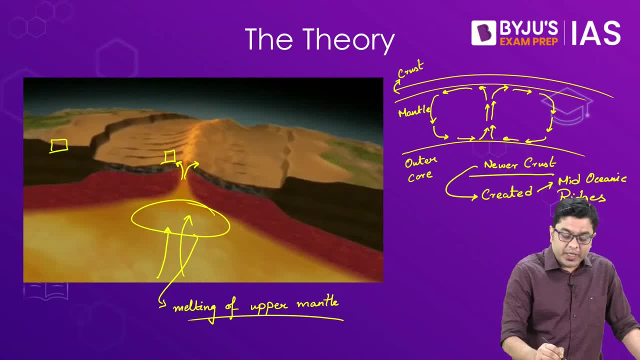 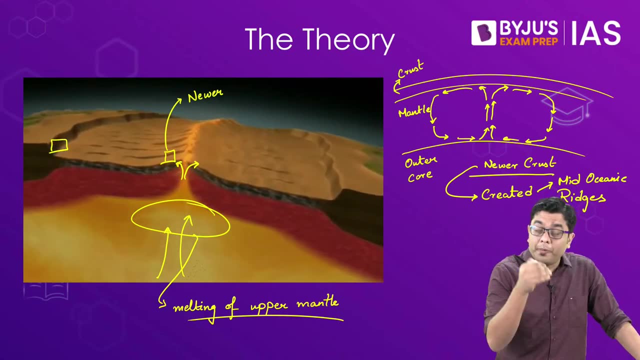 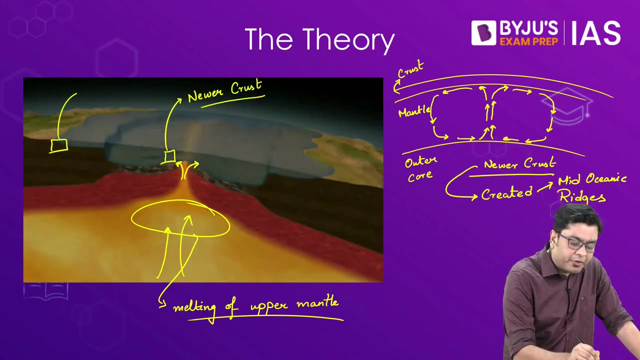 region. immediately in the vicinity of this mid-oceanic ridge, you would encounter newer rocks. So that significantly managed to explain the observation carried out by Harry Hess. So here he would find newer crust and away from it he would find older crust. 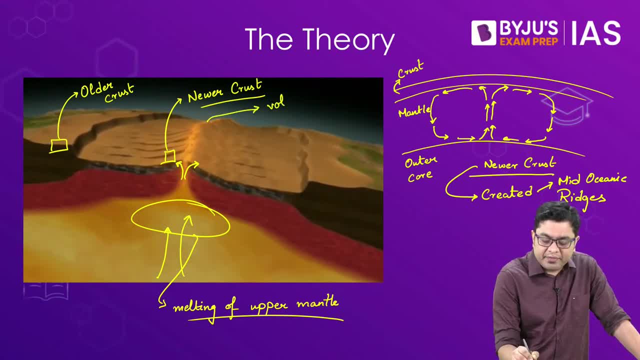 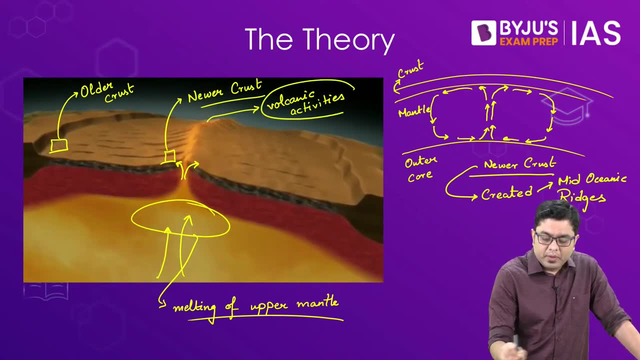 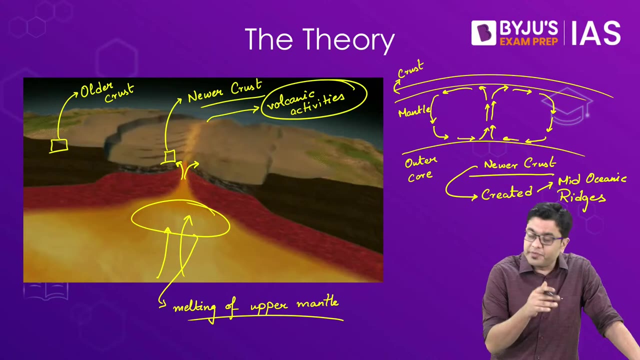 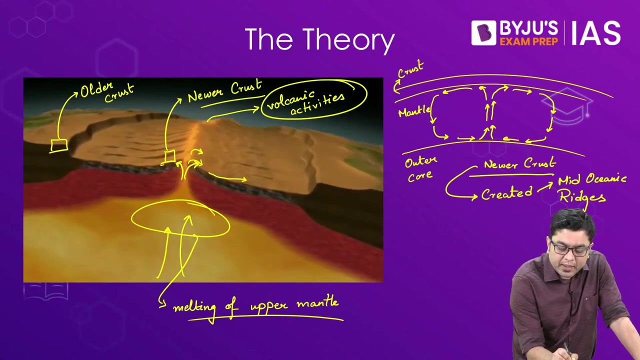 And this was a zone of volcanic activities Now, as you can observe from the animation on your screens as well. basically, when you have the newer crust which gets created, that newer crust, that volcanic eruption that ends up pushing the existing slabs to the sites, But then when you consider earth as a 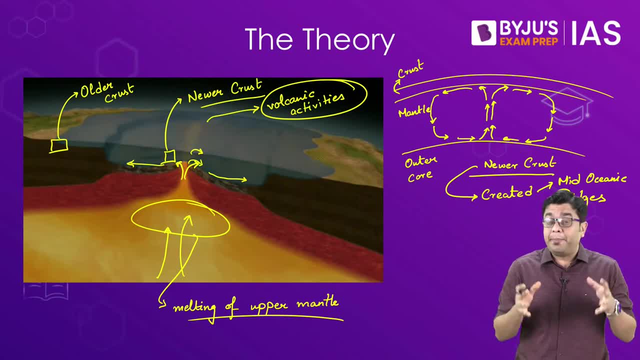 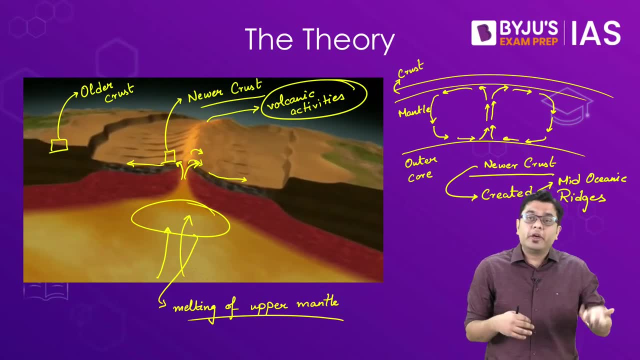 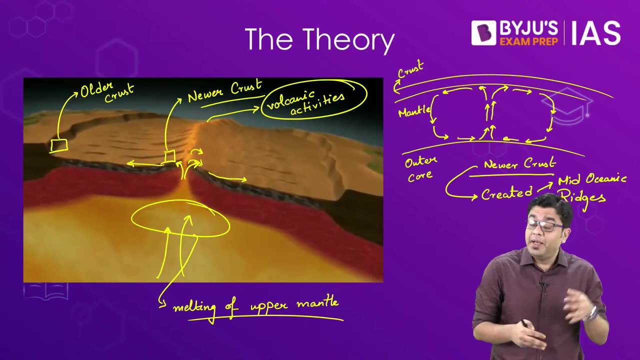 planet. the surface area of the planet is absolutely fixed. It is not changing. It is not as if the surface area or the outer surface, because of this creation of new crust, keeps on increasing. So how is it possible, How is it possible, that simultaneously, newer crust is getting created while the older crust 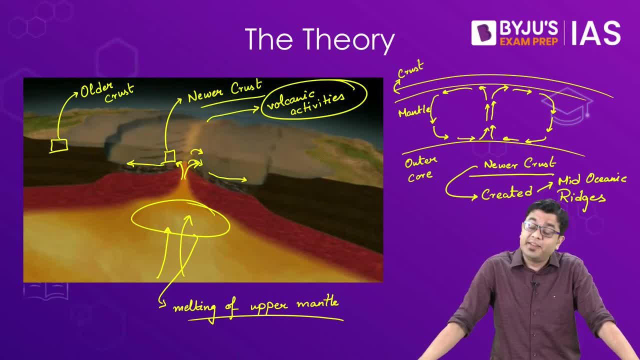 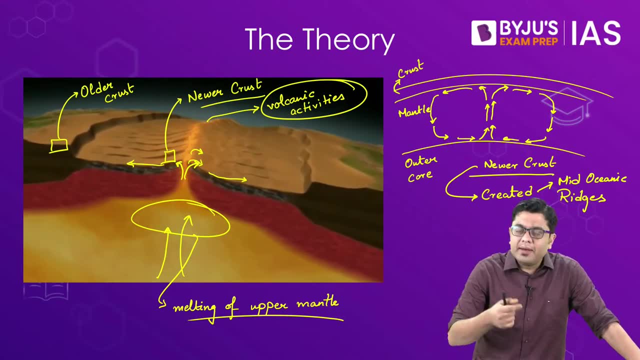 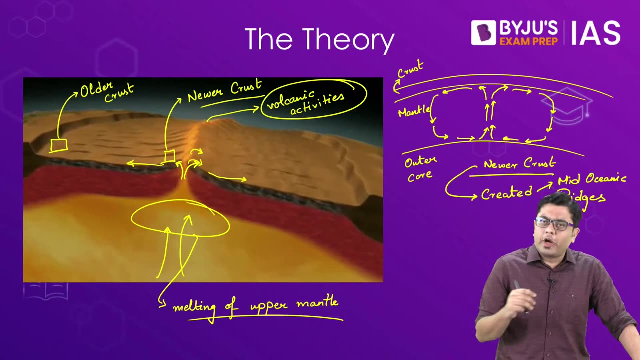 tends to persist in its original form, and the surface area tends to persist in its original form. So that is when Harry Hess again went a step further and provided further explanation for this theory of sea floor spreading. He talked about the recycling of the ocean floor. 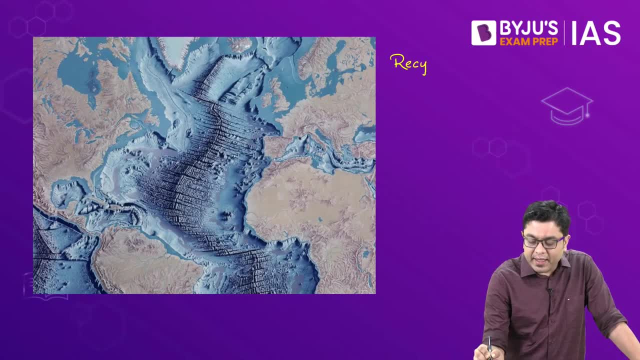 He talked about the aspect of recycling of ocean bottom or the oceanic crust. Now, his postulation was very, very simple. He said that, look, as the newer crust gets created along this mid-oceanic ridge, this picture particularly ends up representing mid-Atlantic ridge, for that. 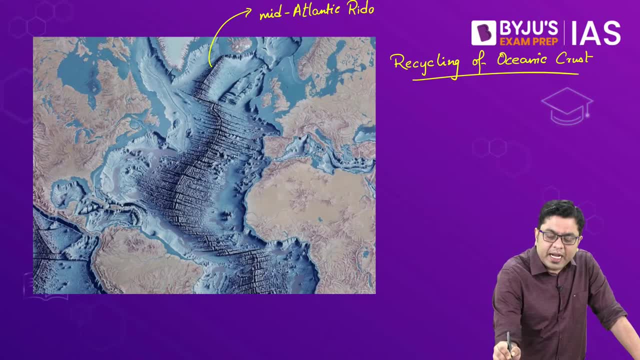 matter. He said that the older crust, the older oceanic crust that gets consumed at the continent ocean boundary and that is where the older oceanic crust simply ends up subsiding and as a result of this subsidence or subduction that leads to formation of oceanic trenches. 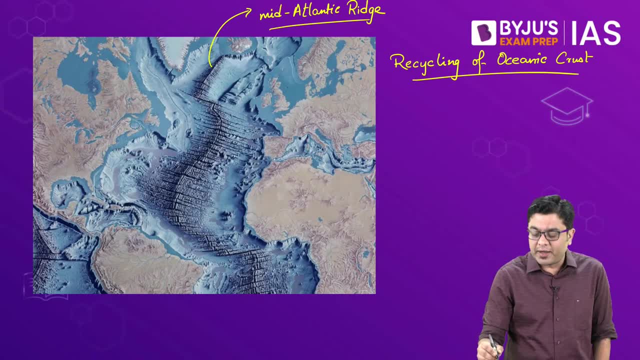 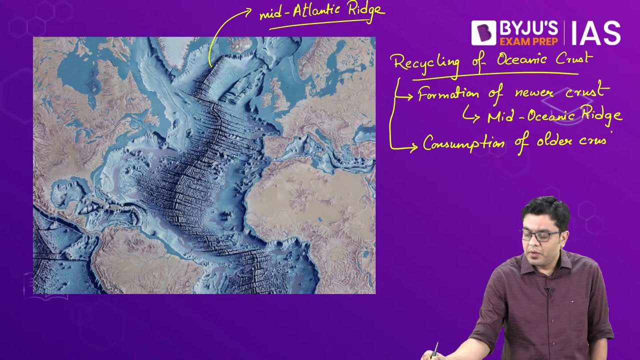 So this aspect of recycling of oceanic crust was represented by the aspect of formation of newer crust: formation of newer crust where, at the mid oceanic Ridge, whereas we had a kind of a consumption of older crust, consumption of older crust observed where, observed at the continent ocean boundary, and this 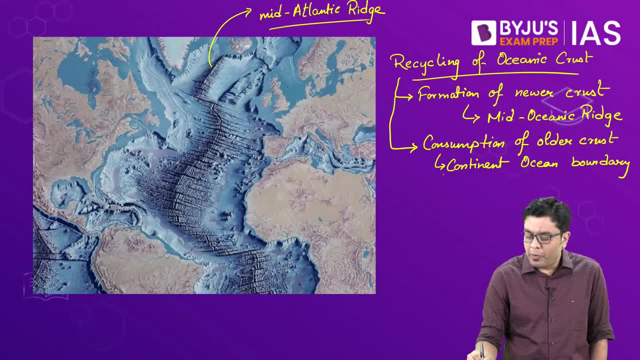 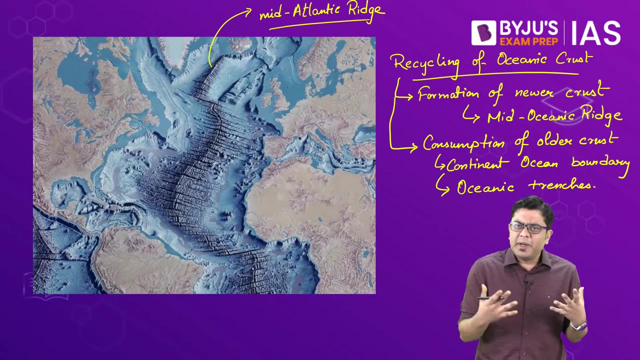 happened, as per Harry Hess, in the form of oceanic trenches. so if you have to think about the diagrammatic representation of the entire oceanic boundary at the mid oceanic Ridge, if you have to think about the diagrammatic representation of the entire entirety of the theory, the diagrammatic representation will also be quite similar in the sense that 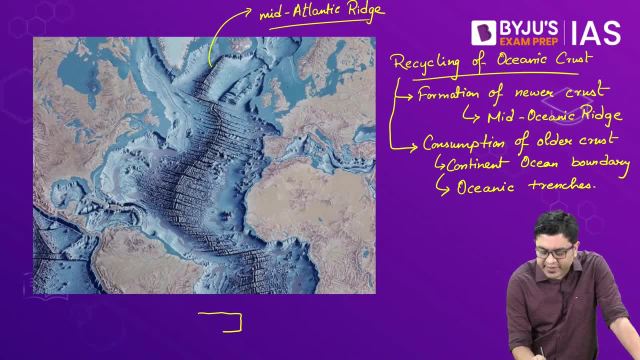 if you have, let's say, a continental crust on the sides, a very basic diagrammatic representation that I am talking about, and in between them, let us say, you have the oceanic water. ocean water, now the sea floor overall would represent. as per this theory, sea floor would represent. 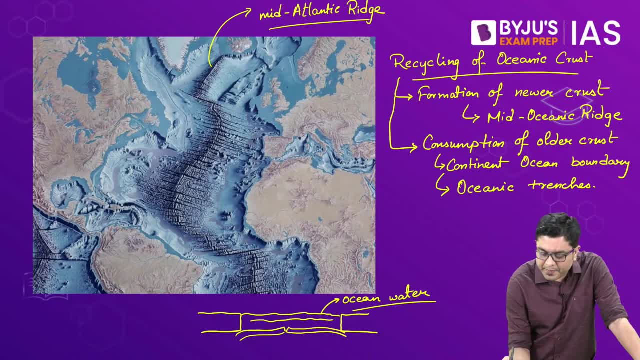 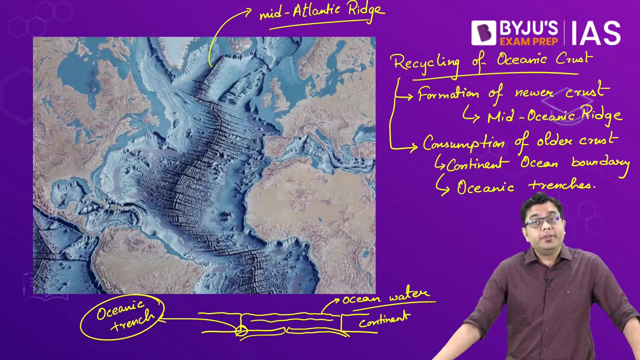 a kind of an existence somewhat like this, and there at the continent ocean boundary, this being the continent and this being the ocean floor, so at the continent ocean boundary, you had the oceanic trench where the older crust would get consumed. so this entire cycling process by that. 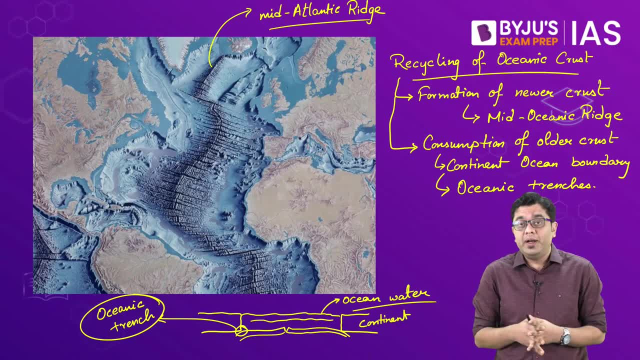 Harry Hess could talk about and talk to the whole world that look. this is the reason why along the ocean bottoms we don't find any part of the sediments or the rock system which are older than 200 million years, because after a small amount of time, 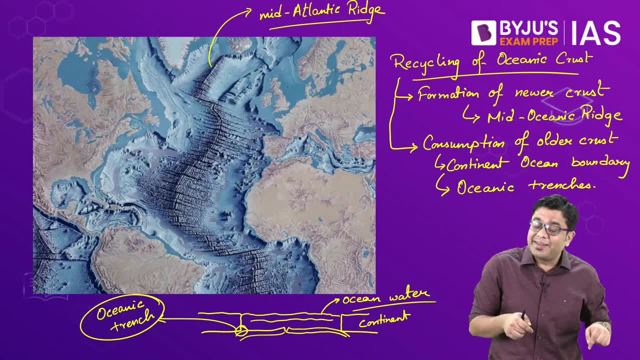 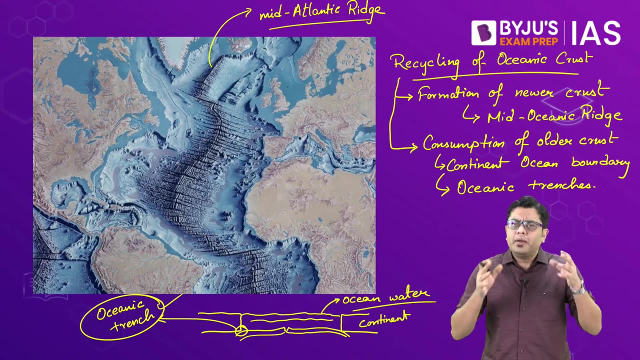 all of that oceanic floor that gets subducted underneath the continental crust and creates this oceanic trench. so this was the aspect of sea floor spreading. this was explained by Harry Hess. this particular theory in itself had certain limitations, but then it also proved to be significantly helpful in 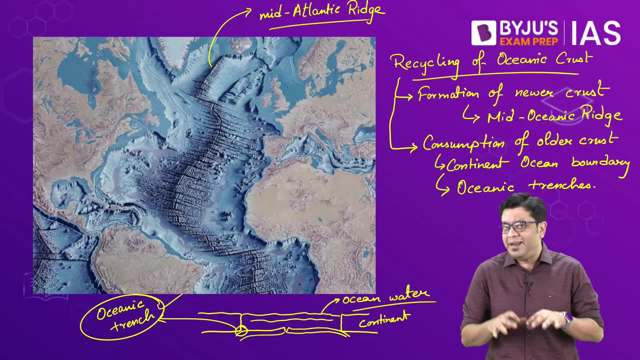 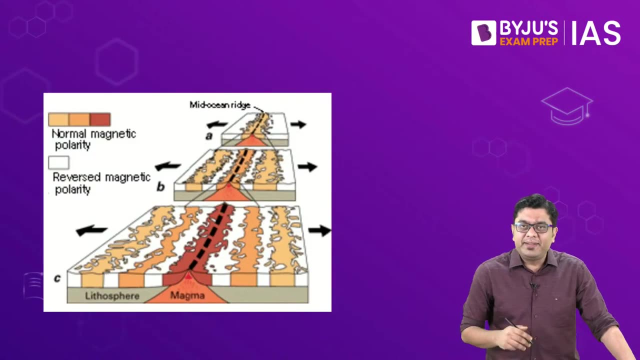 postulation of newer theories, as we will look at later now. along with these there were other evidences which could support the aspect of sea floor spreading, but that was not exactly propounded by Harry Hess himself and that evidence was something which came to light and that was the aspect of paleo magnetism. now, 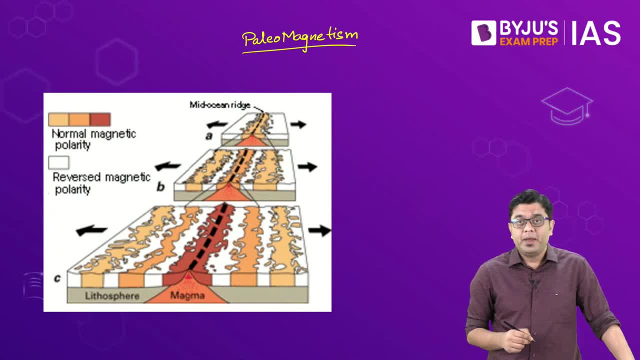 what is this aspect of paleo magnetism? you? this was basically understanding the age of the rocks depending upon the magnetic field lines that the rocks indicated. now, paleo magnetism basically helps us understand when is it that a rock would be formed, how, so we know that the 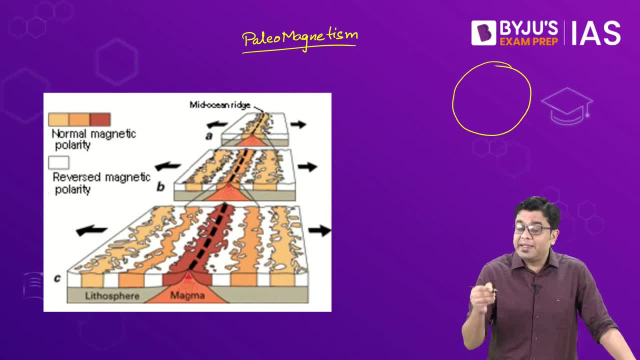 entirety of the planet. overall, the entirety of the planet ends up behaving like a magnet, like a bar magnet, and you basically have the magnetic field lines which originate from the magnetic north and the south poles. but then this magnetic field line is not often fixed, it keeps on changing. 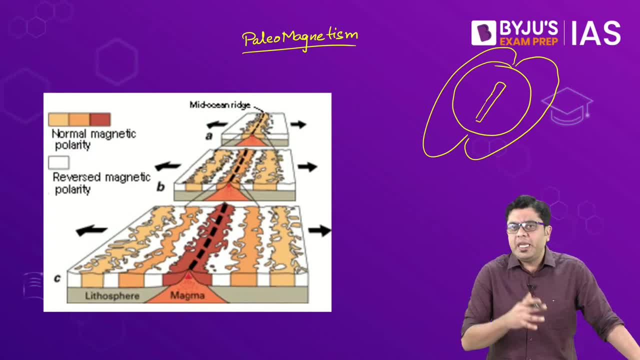 as is and is prone to various changes which keep on happening. now suppose a rock gets created. so a rock will be created by what process? by the process of volcanic eruption. so when there is a a volcanic eruption which ends up creating a newer crust, so that means lava would cool down. 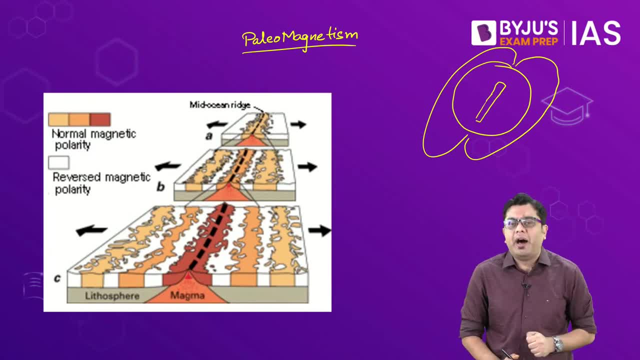 but during that process of cooling down of lava, the particles in the molten form, they align themselves with the existent magnetic field observed across the planet at that point of time. so by studying and analyzing the magnetic field lines exhibited by the various rocks, we can very easily end up calculating the age of the rocks. so this was initially the study was. 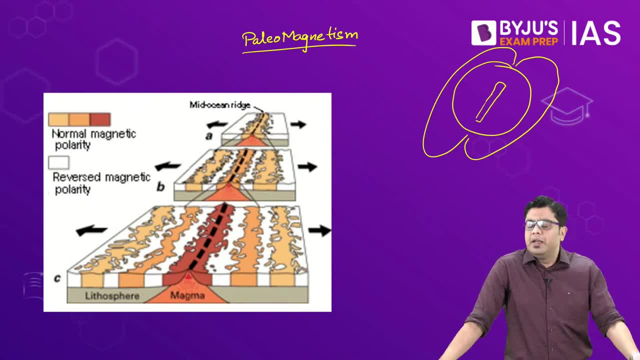 carried out and introduced by harrys himself. now he studied the pacific flow of the coastline of california and there, when he was carrying out his study, he observed certain magnetic anomalies. magnetic anomalies in the sense that on one side of the mid-oceanic ridge he observed that every 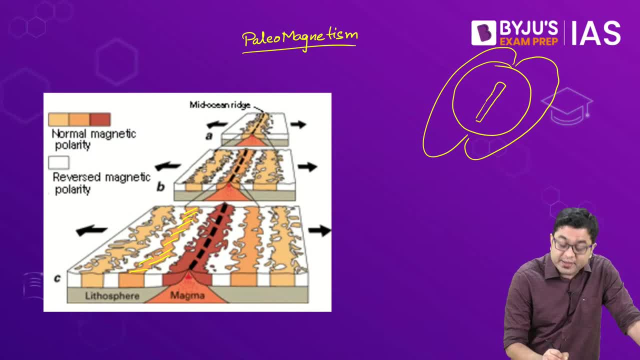 few distance. every small distance ended up representing a different kind of magnetic behavior. that did not make much of a sense to him. but then when the other portion and the other side of mid-oceanic ridge was studied, that is when people found a kind of a similarity. they found the similarity. 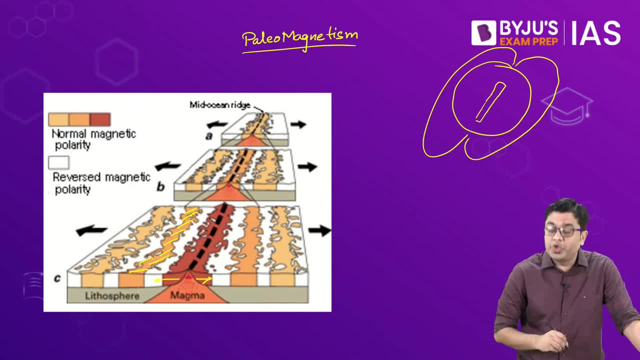 that when you start moving away from this mid-oceanic ridge you end up finding rocks having and indicating a similar magnetic property and that similarity was very stuck. so as you move a certain distance away from the mid-oceanic ridge you find a kind of a similarity in the magnetic 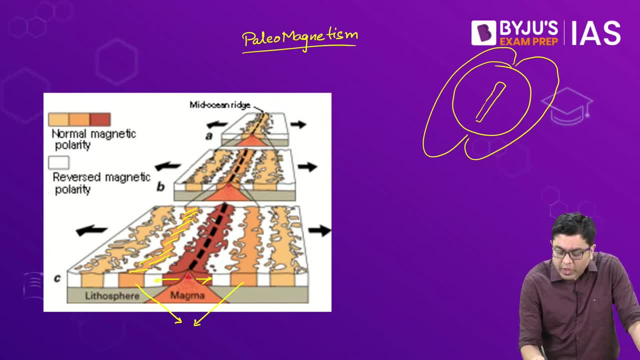 properties, which again indicated that the rocks along these lines would have had same time period of origin, of origin of paleomagnetism, which further reinforced the concept of seafloor spreading and further strengthened the idea that there is a crustal recycling going on and you have volcanicity. 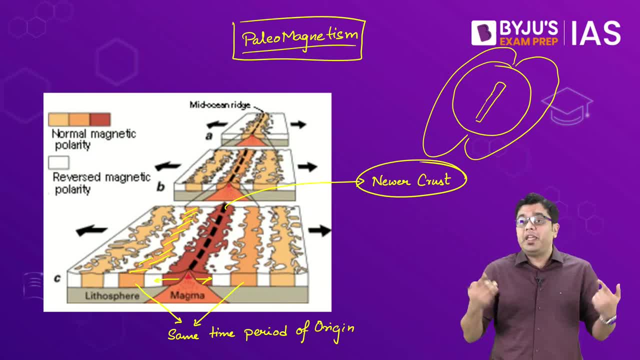 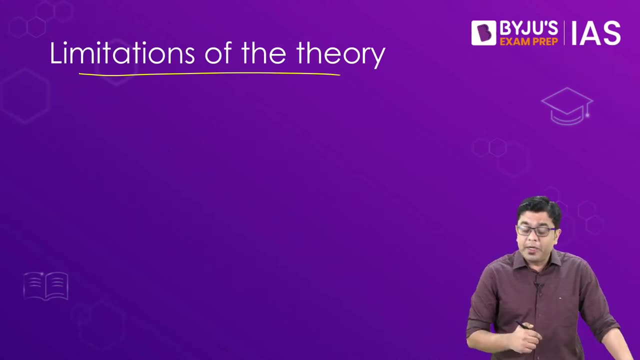 being one of the major factors leading to the creation of the newer crust. Now, this particular theory also had certain lacunae and certain drawbacks. So if you talk about the limitations that were highlighted by this theory or which came into light because of this theory, first limitation was that this theory did not talk about the movement of continents. 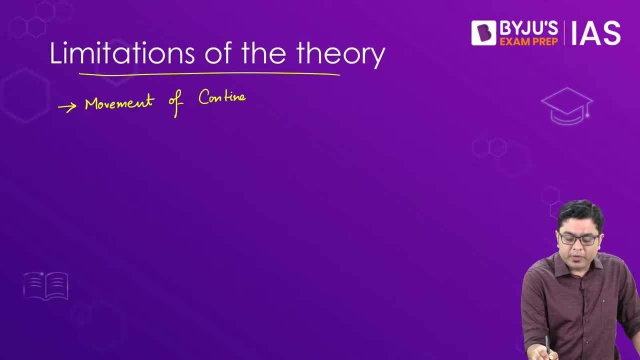 Movement of continents was not talked about by this theory. It did not talk about the aspect that the continental landmasses could move as well. It talked about the aspect that, yes, in the seafloor, the ocean floor, gets reclaimed, But then what is the impact that it will have on the continents? Are the continents moving as well? 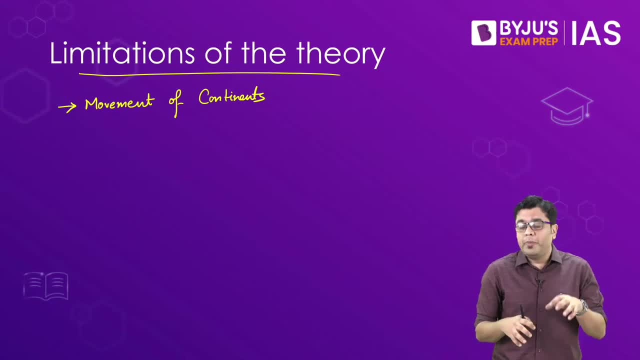 As we know now that all the continents, they are also perpetually in one kind of motion or the other. If we take a look at the continental landmass of Indian subcontinent, it is consistently pushing into the Eurasian landmass, further accelerating the height of the Himalayas. 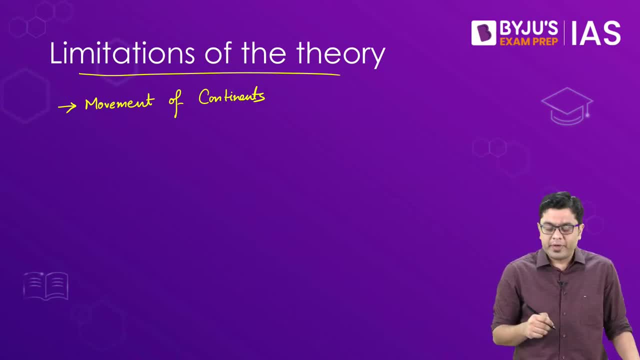 But then seafloor spreading did not talk about it. Then the seafloor spreading, While it carried out a study of the ocean bottom but could not explain the formation of various relief features in existence at the ocean bottom. So it could not and did not explain the features of ocean floor. 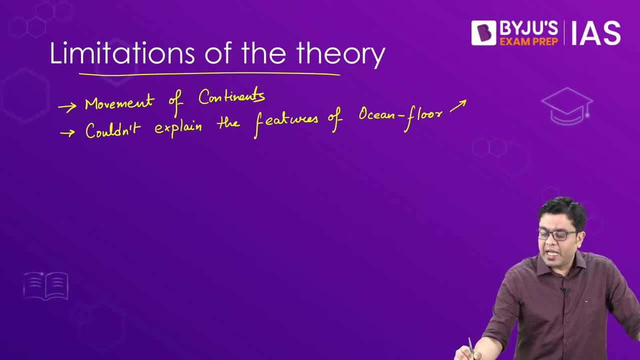 which features are we talking about? We are talking talking about the aspect of seamounts, goyards, etc. So these were left unexplained. But other than that, there was another major flaw which was present in the theory of seafloor spreading. 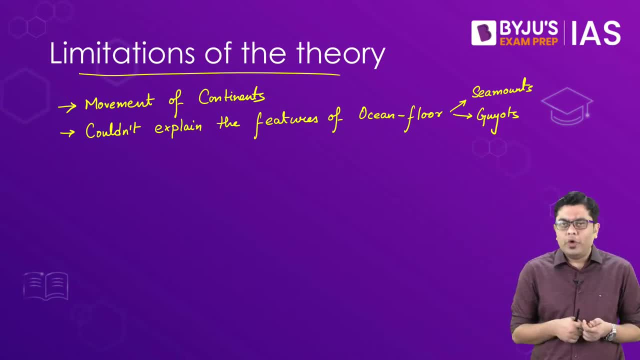 Now seafloor spreading talks about the recycling of the oceanic crust. As per this theory, wherever you have the mid-oceanic ridge, at all these oceans, along the boundary lines, you need to have the existence of an oceanic trench, so that that would end up advocating that yes. 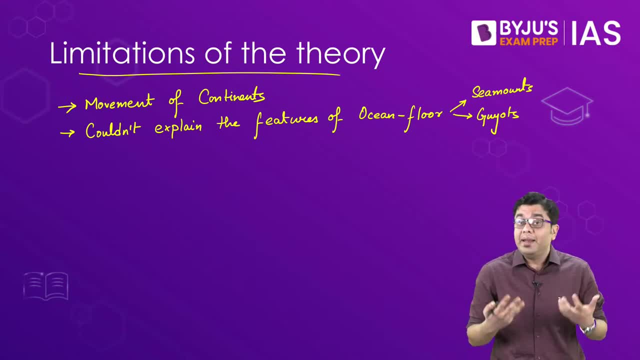 the older crust is being consumed. But then that did not come into reality. So, as per this theory, each and every ocean continent boundary should have the existence of an oceanic trench. only that would support the theory that, every time and everywhere that seafloor. 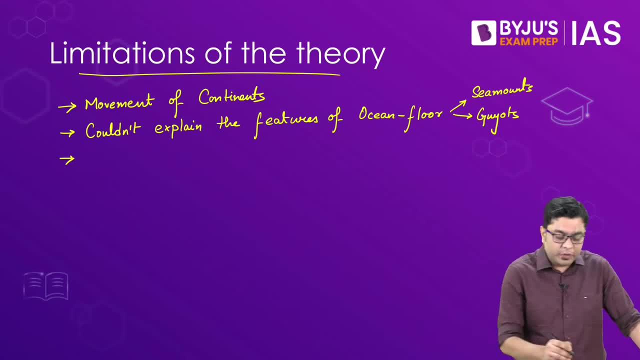 that newer crust gets created, the older crust is consumed. So could not explain the lack of oceanic trenches where, at every continent, ocean boundary, because these oceanic trenches, they are not to be found everywhere, they are found only in certain locations. later, with the various different theories which came into existence after this, 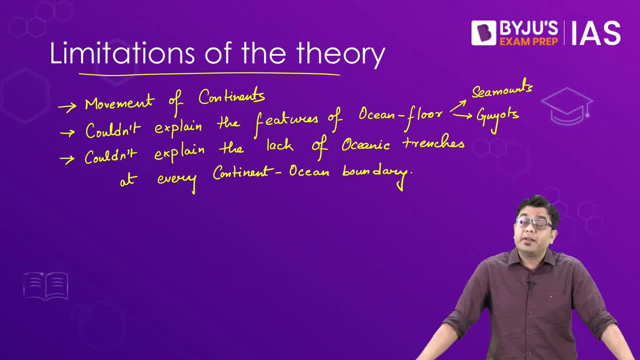 we know now where these oceanic trenches can get created and why do they get created, and that is explained by theory of plate tectonics. but then at this point of time, this theory could not explain that. why is it that along the boundary region of atlantic ocean and north 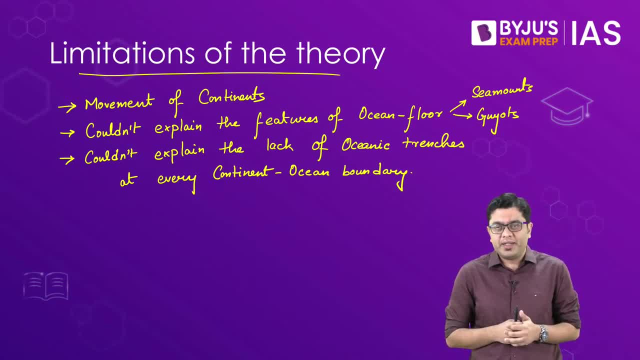 american continent, you don't have a large oceanic trench in existence. similarly, along the boundary zone of european landmass, along with the atlantic boundary, you don't have a large oceanic trench in existence. so these were certain drawbacks and limitations of this particular theory, but, having said that, this theory nonetheless proved to be significantly important. 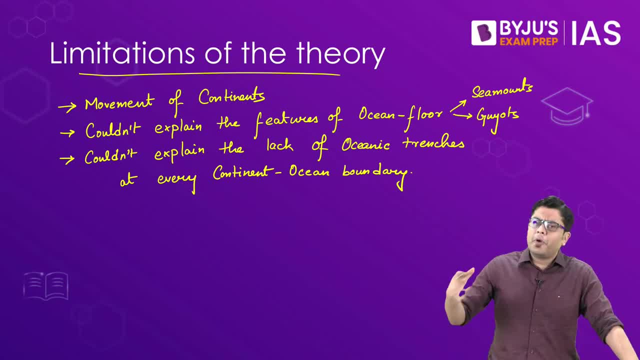 and was a landmark in the sense that it provided a concept and a kind of a linkage between the earlier propounded theory of continental drift, which was provided by alfred wagner, which talked about the movement of all the different landmasses, and the future theories which could explain it all. 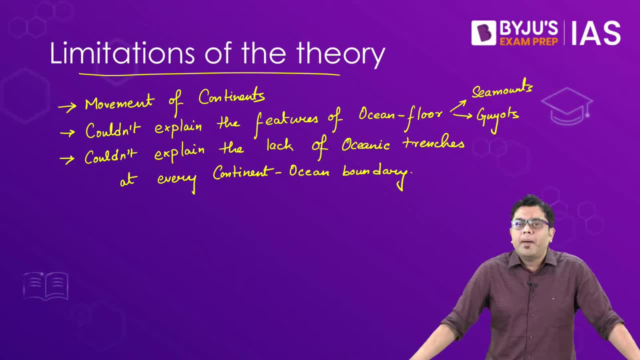 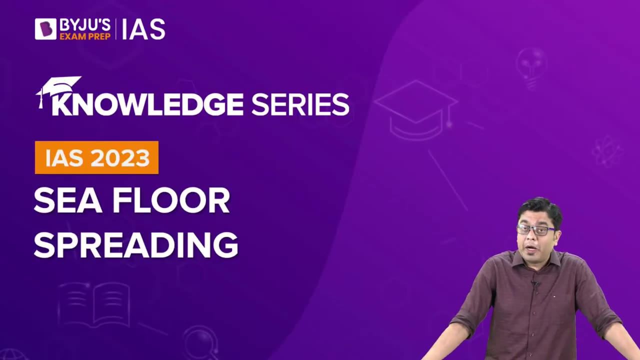 that is, the theory of plate tectonics. so scientists and geologists such as mckenzie, parker, etc. they used this in order to explain the plate tectonic theory which came into existence. so, basically, if you have to talk about the seafloor spreading theory, while it significantly accelerated our understanding regarding the earth's 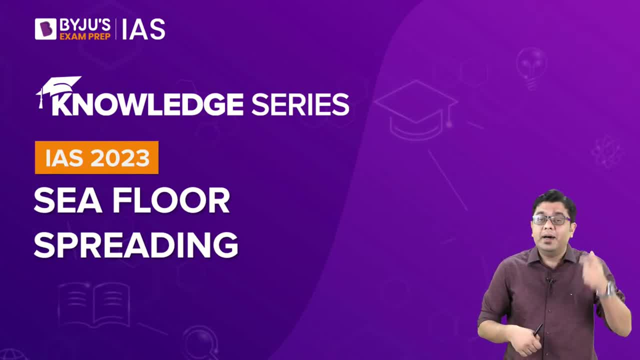 lithospheric land mass and what happens underneath the earth's crust. it also helped us understand why is it that areas such as atlantic ocean they are expanding, whereas areas such as pacific ocean they are and declining in size And, more importantly, it helped us provide a framework for the newer. 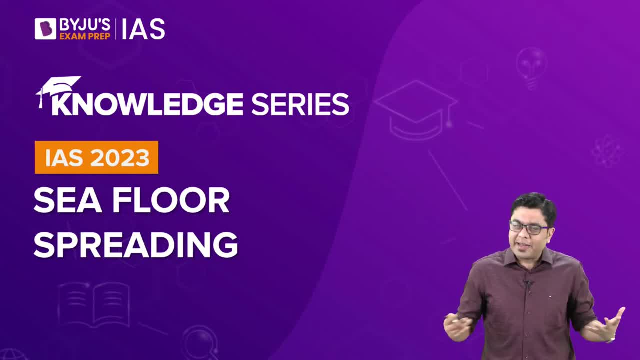 acceptable theories in existence. So that is all that you need to know about the theory of seafloor spreading. This can always be important in the form of direct questions which have been framed from there in the UPSC mains examination, where a candidate is supposed to explain all. 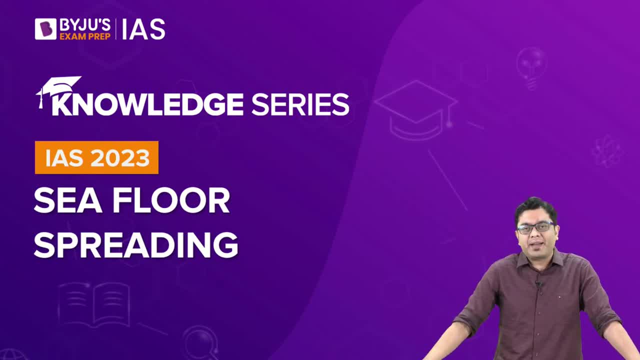 these observations and evidences, along with the drawbacks and the benefits and advantages that this theory held for us. Now, having said that, and before taking up the questions again, let me reiterate that particular announcement that now we have covered more than 100 sessions of the. 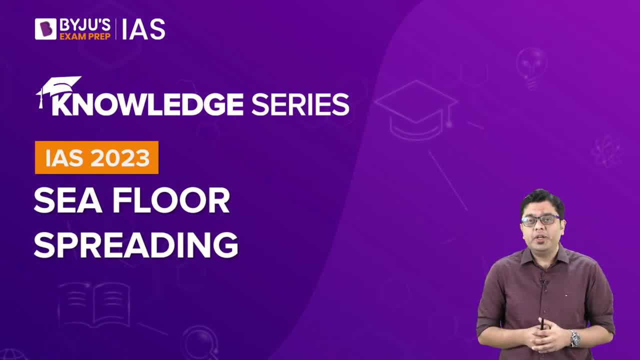 knowledge series. This and today's session marks an end to the weekly episodes of knowledge series. From next week onwards, we shall be having a series of knowledge series, This knowledge series being held on the weekends, where we shall be having one session each on the. 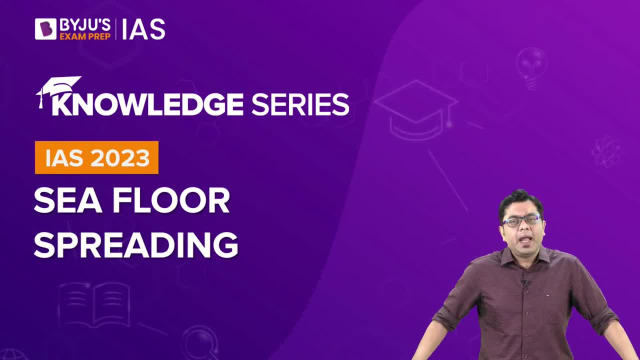 weekend, and there the announcement shall be made and accordingly the schedule shall be circulated. Now let us take a couple of questions. So a question by Pavitra: does paleomagnetism vary to the old crust formed away from the mid-oceanic ridge? Yes, the magnetic property ends up changing. 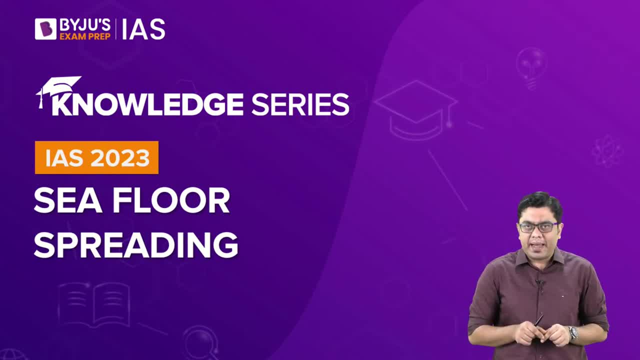 and that ends up indicating a kind of a similarity. That indicates that, let us say, you are moving 50 kilometers away from the mid-oceanic ridge, on either side. Both of these, if they have a similar magnetic property, a similar magnetic anomaly, then that indicates that their age of formation. 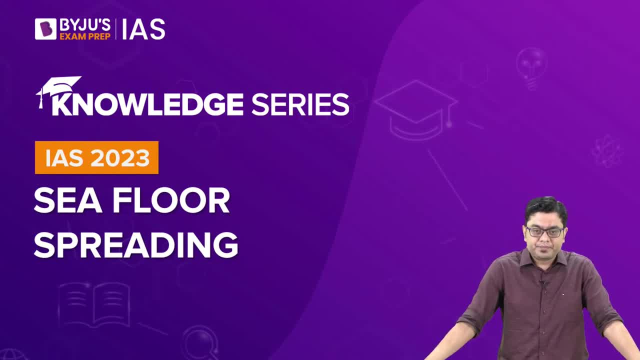 would also be the same. Okay, One other question that what kind of question UPSC can ask from here. So UPSC has been known to ask a direct question from it in general studies means as well as in optional means where the question is. 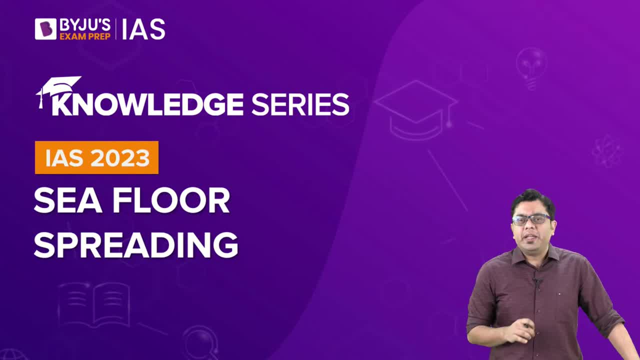 very direct. The question is: what do you understand by the theory of seafloor spreading? Highlight the advantages as well as the limitations of this particular theory, Raj, in order to make notes of it. you just have to talk about that: what this theory is. 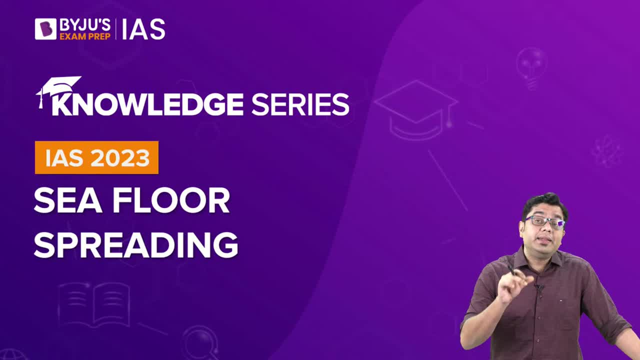 who postulated it. You have to bring into light slightly the convection current theory provided by Arthur Holmes and that explains the volcanicity which is observed across and along the mid-oceanic ridges and how the creation of a newer crust pushes the older existing crust to the higher. 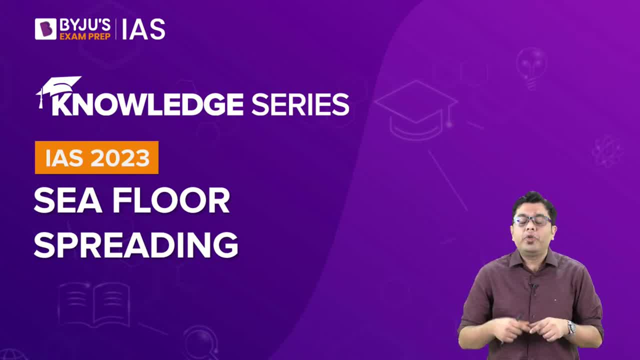 to form the trenches. After that you have to talk about the evidences which supported, the evidences in the form of seafloor spreading and the evidences in the form of paleomagnetism That needs to be highlighted, And after that you have to push forward the limitations. 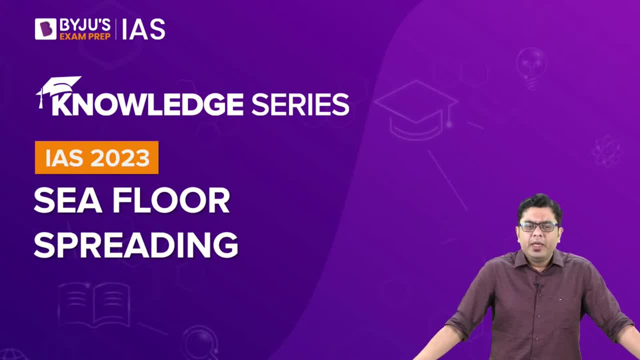 Santosh Kumar regarding the plate tectonics, So the theory of plate tectonics. it basically talks about the fact that the entirety of the Earth's lithosphere- And when we say Earth's lithosphere here, please understand- Earth's lithosphere talks about 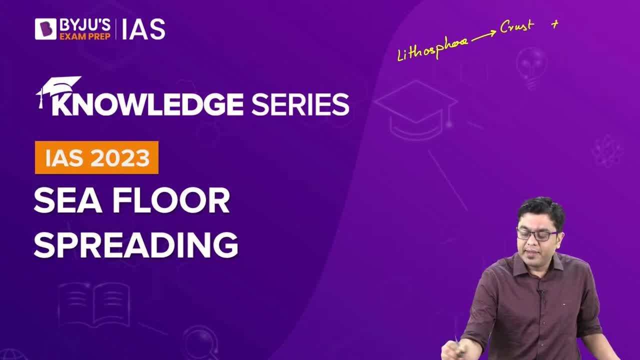 the portion of the crust plus the solid part of upper mantle. So, as per the theory of plate tectonics, the entirety of lithosphere that is broken and it is divided into various different particular subunits, different plates, and those plates end up moving with respect to each other. and as they move with 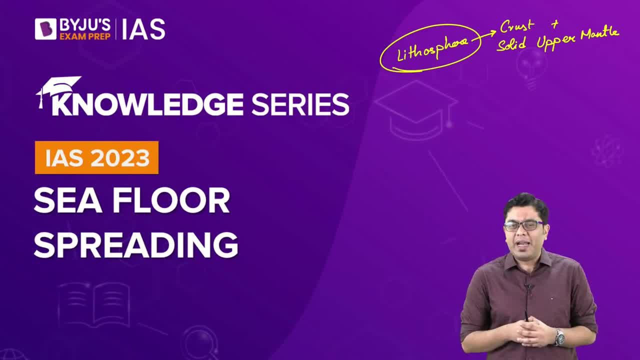 respect to each other. that leads to creation of newer land masses and newer geological features and geographical phenomena, such as volcanism, as well as seismicity, which is observed in many of these plate boundary regions. but then the movement of these plates is again something which is initiated because of the immense amount of heat which is present in the interior of the earth. 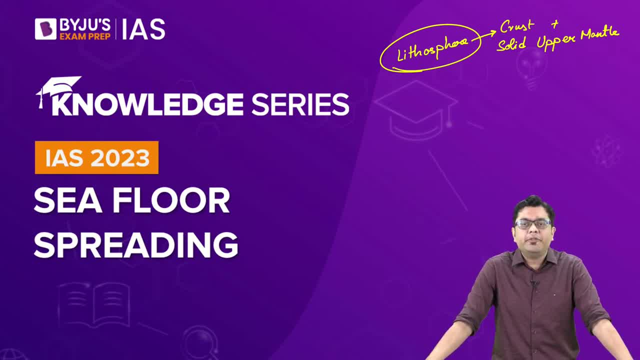 and that heat travels to the exterior in the form of convection currents. okay, so that is all, and that is where we conclude this session of knowledge series. we shall meet again on the weekends thereafter. if you like this endeavor of ours, please don't forget to click upon the like- share. 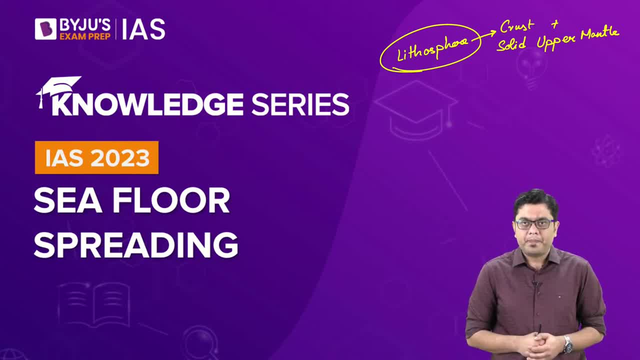 and the subscribe button. thank you you.